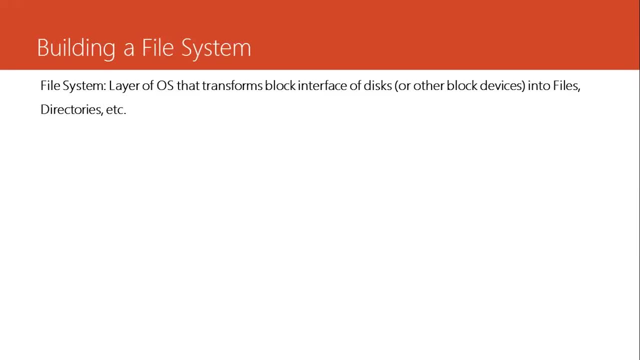 a file system? Well, it's a layer of operating system that transforms blocks into files and directories. okay, Blocks are not something you deal with as a user. You don't think about a block. you think about files and directories, right? So some components of the file system are things like: what's the disk management? 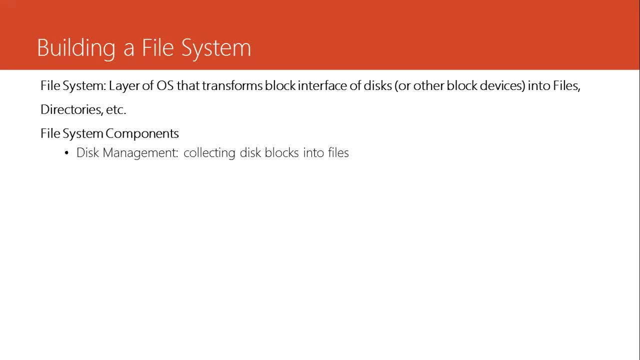 This is the component that is responsible for collecting disk blocks into files. naming of files. How are blocks put into files so that the user only has an interface to files by name rather than by blocks? When you find a file, you usually find something like user slash home, slash some file. You don't search by blog. 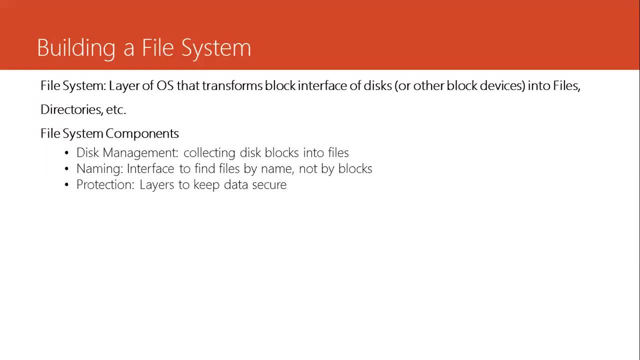 right. and then, how is our data kept secure and How is our data kept reliable and durable? keeping of files durable despite crashes, media failures, virus attacks, Etc. These are important questions to address while developing a file system right. Then there is also the user versus a system view of a file. 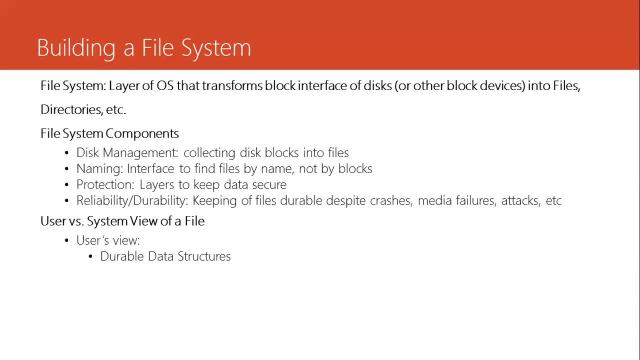 So the users view of a file is a bunch of durable data structures, Whereas the systems view of a file is a collection of bytes, and it does not really matter To the system how the user is using those bytes. Okay, the system thinks of it as a collection of bytes. and then we also have the systems, you inside the operating system. 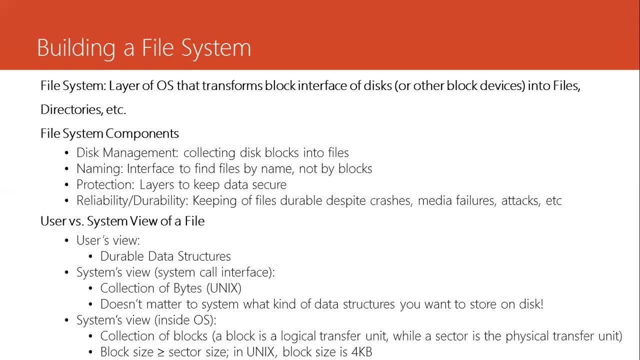 Which is the collection of blocks, and blocks on the operating system side are viewed as file fragments and the blocks on the physical disk are the sectors. Don't forget that block size is greater than or equal to sector size, Because a sector is a block for the physical disk drive. 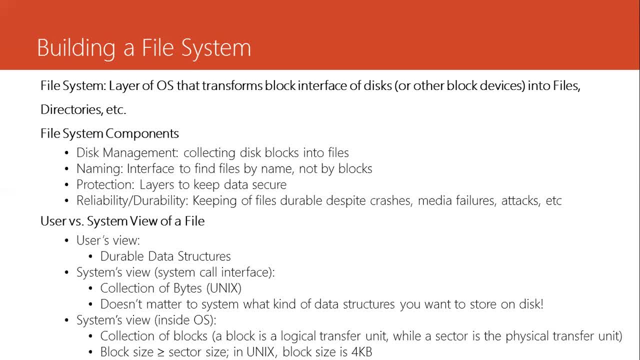 However, the operating system could combine a bunch of these blocks and name it a block. So when we talk about the block, it could actually be more than one sector. We talked about this in the first video. Okay, so there's a bunch of different ways of looking at a file and we are going to 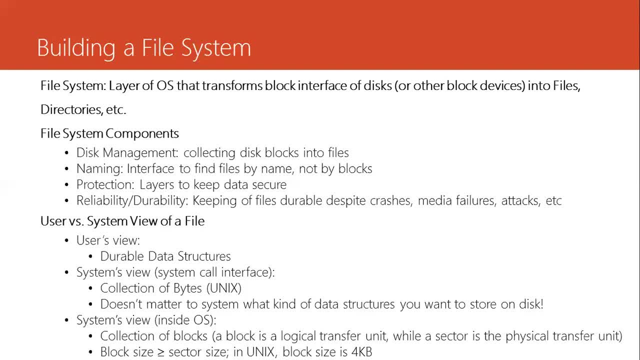 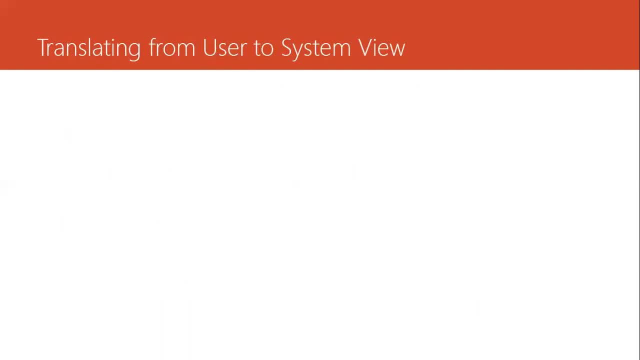 have to make sure that We take all these aspects into account when we design our file system. So here is the is the process of translating from user to system view. the user view is a durable document and somehow the file system has to turn that into blocks on a disk right and 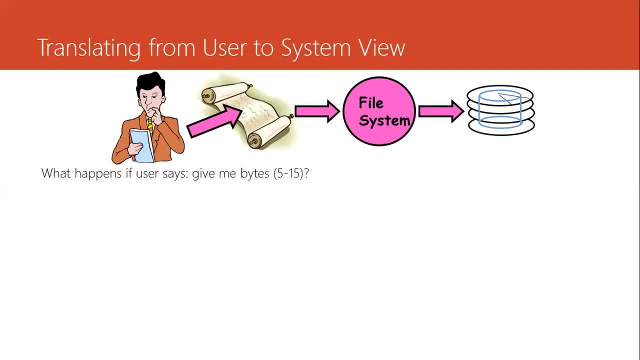 What do you think will happen if the user requests for certain bytes, Let's say 5 to 15.. What is the file system going to do? first those blocks of the disk into memory, Extract these bytes and then hand them back to the user. Okay, and what does that mean? Well, that means 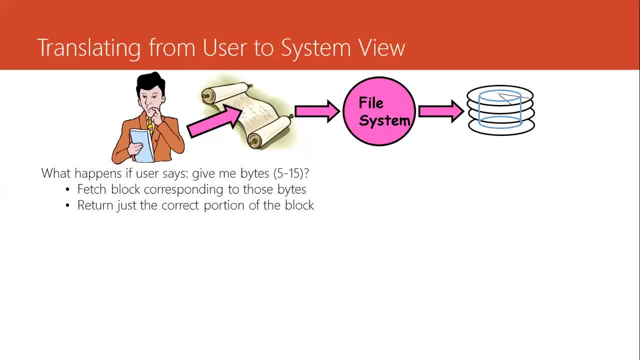 there's got to be some some sort of buffering inside the file system. and More interesting is the case of right, For example, if I say, write certain bytes into a file, in that case We have to load the blocks of the disk, Then fill in the required bytes and finally write the whole block back to the disk. 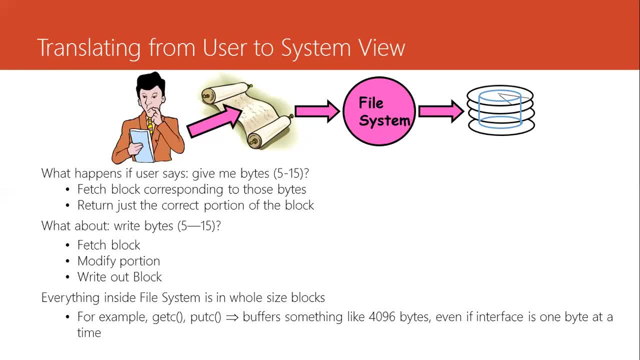 Because the only interface we have to a disk is a block interface. There's a lot of caching inside the file system and there is quite a possibility that you write your data into the file And it's not yet on the disk before the system crashes. Okay, so that's something to worry about. 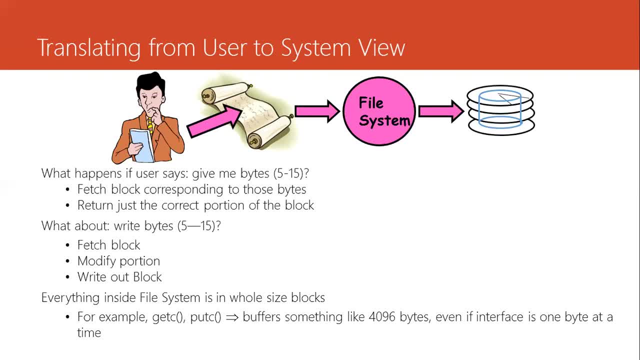 Everything inside the file system is in whole size blocks. So for instance, get C and put C basically might buffer up for you 96 bytes or 4 kilobytes before writing it out, because disk drives have a block interface and not a byte interface. From now on, a file for us is basically a collection of blocks that we are going to somehow organize into a file structure. 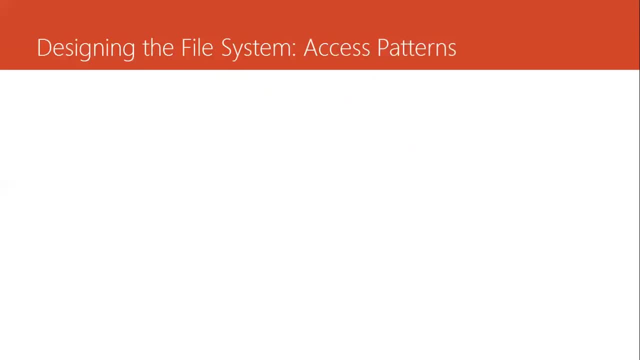 Okay, Let us discuss very briefly some access patterns that Have been observed over years of analysis. How does the user access files? So while designing a file system, you need to know the kind of access patterns the user is likely To throw at the system. So we have two kinds of access patterns. 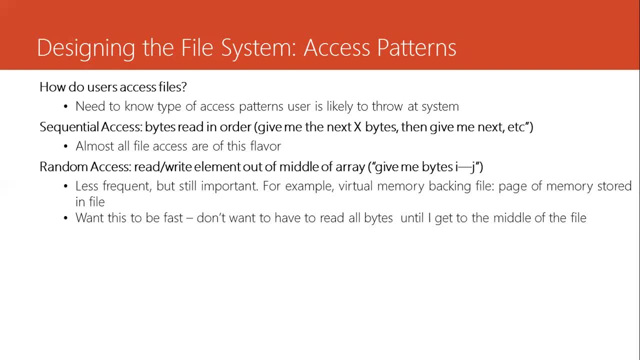 Sequential access and random access. observations have indicated that That almost all file accesses are sequential. Sequential accesses are placed in contiguous blocks. on the other hand, random accesses are less frequent, but still important. Then there is another access pattern that is content based. So the file system also must be able to search based on the content of what the user needs. 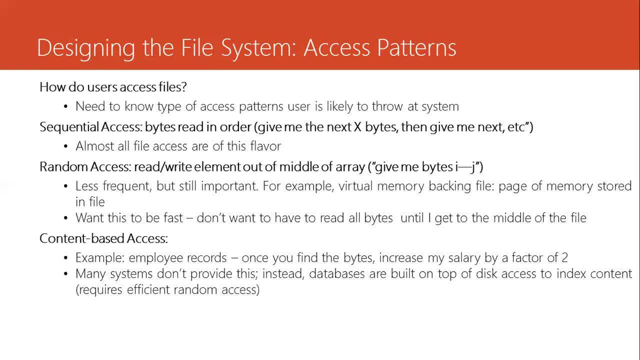 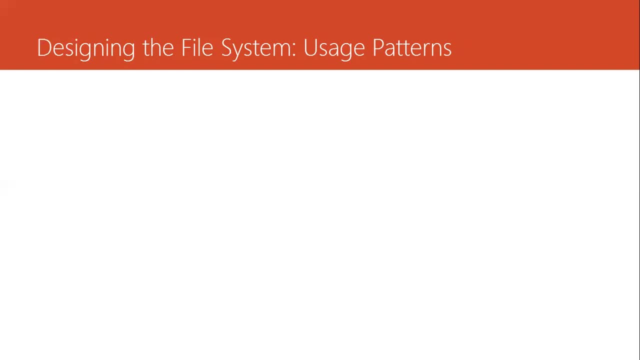 Although many systems employ databases that are built on top of this access to index the content. that, however, requires efficient random access. The designer of file system Must also be aware of these usage patterns. So how does the user actually uses the system? What sizes of files users you usually have? Okay, 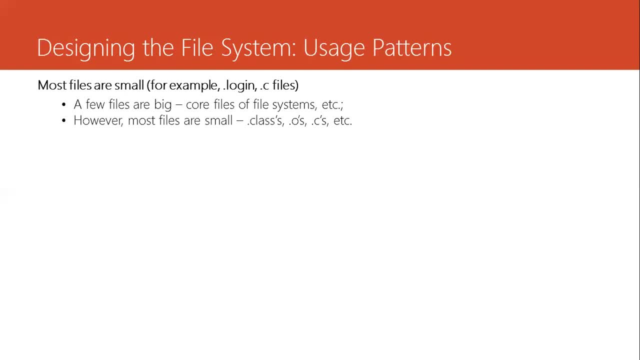 usually Only a few files are big. that uses much of the disk space and bandwidth to and from the disk, and most of the files are small. a five years of Facebook Has also highlighted this fact: that most of the files are small, But most of the space is used up by the rare big ones. 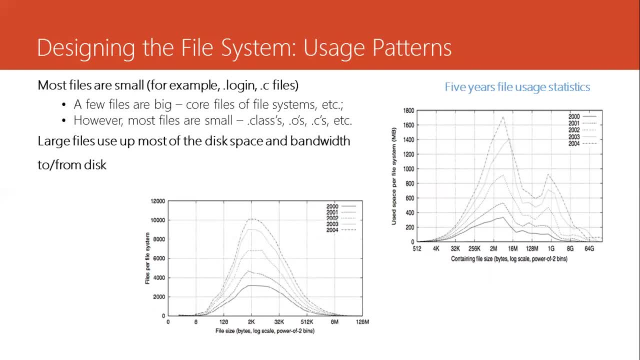 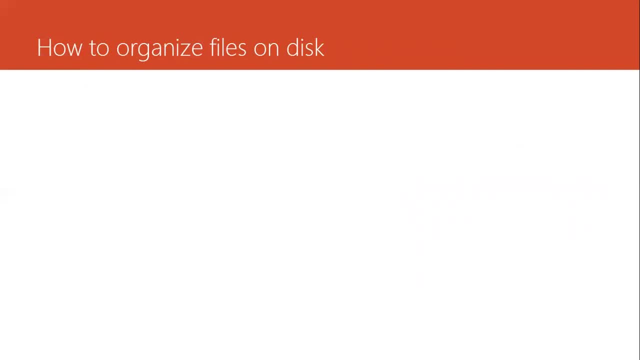 So our file systems need to have support for big files as well. so the million dollar question is How to organize the data. well, These are some of the natural things, or the kind of support that any file system should provide, and before the user right one one: we want to maximize sequential access, so we want to 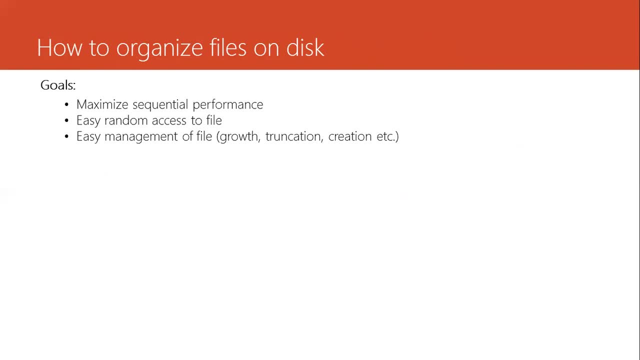 maximize sequential performance and to random access must be easy as well. yeah, and three, we must provide easy management of files. it must provide some way to edit files in a way to grow or shrink the size of the file files. right, because you edit files all the time. okay, so essentially this interface would give: 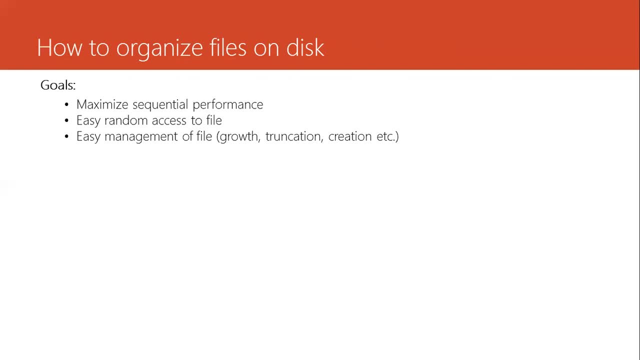 the user a simple view of files and directories and the file management system actually would map or allocate these files and directories into sectors on a hard drive. so one of the ways to do this allocation is by contiguous allocation. that is one of the simplest things one could do. so what do you do? 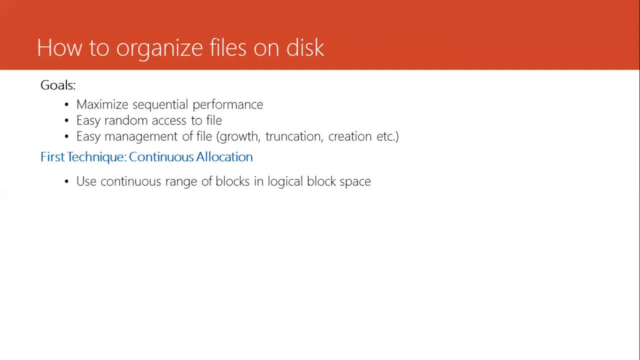 you use a continuous range of blocks on on the disk and every file has to be contiguous, non broken group of blocks. let's assume that we have this file and this is our disk drive, with data blocks represented by the small boxes. these small boxes are the actual physical sectors on the disk. to simplify things, we have led those. 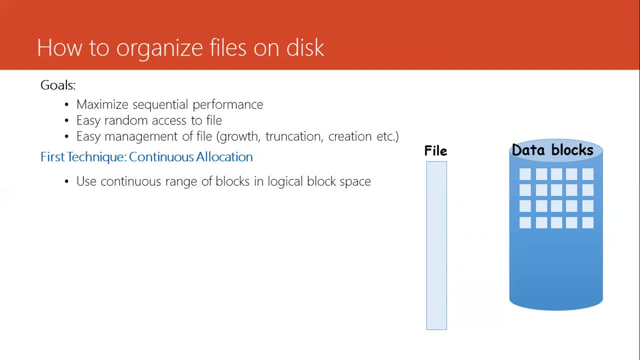 sectors in this manner. okay, one of the responsibilities of the file system is to break up a large file into logical blocks that is equal to the size of a sector on the disk, and then the file system needs to map all these files onto sectors of a hard drive in a way that is. 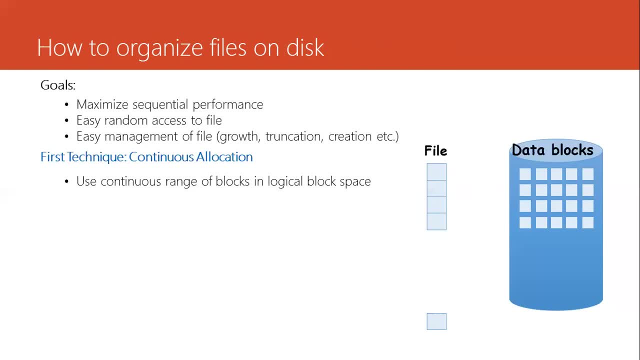 efficient so that the user could access their files with ease. so in the case of contiguous allocation of these logical blocks, we need to find a free range of blocks large enough that fits the data completely. one way to implement this method is that we might have a bitmap of 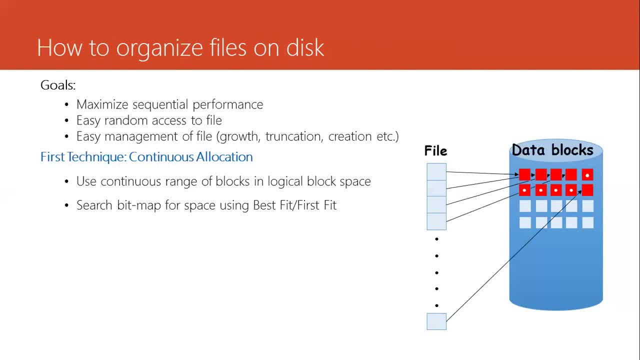 free space and what we need to do is find the biggest chunk using best-fit or first-fit algorithms. we also have a video on best-fit- first-fit algorithms. when we get to the memory management module, that addresses a special region of memory known as heap, where all your runtime dynamic variables resides. for 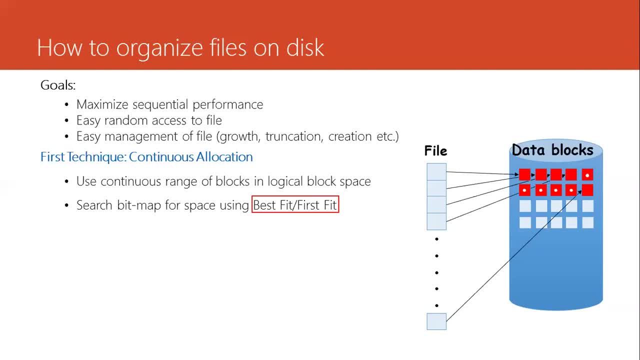 now just briefly, the best fit and the first with algorithms are used to search for a free range of blocks based on theAlgorithm and the first-fit algorithms used to search for a free range in the available free space to fit the file in that contiguous location. on this, 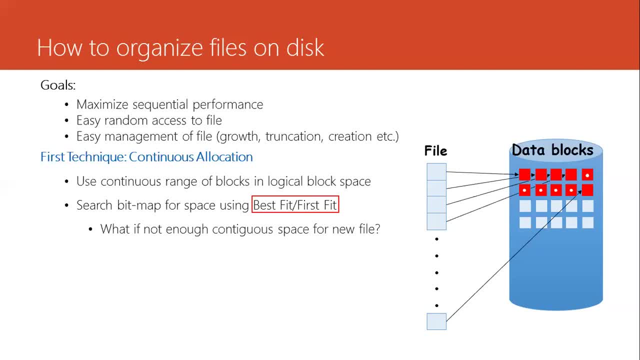 so, coming back to our discussion, what if there is no space available where the file fits completely? then we will have to move the file around to find a place where it fits, and you might imagine how expensive that would be right, okay, so what's the great thing about this matter? this method has the best sequential 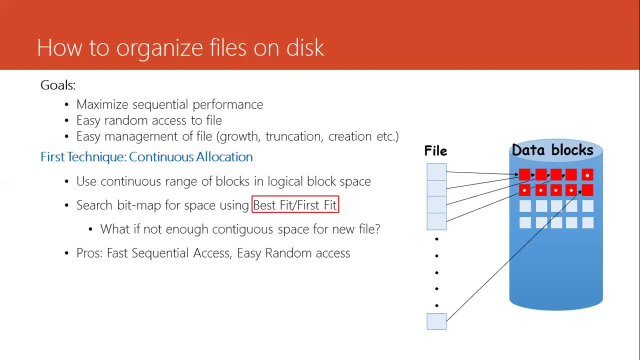 performance because you place the head in one place and you just spin the disk and you get the whole file right. so this method has fast sequential access and easy random access as well. why is it random access? because you have this starting address and you can always add the offset of the block locations you 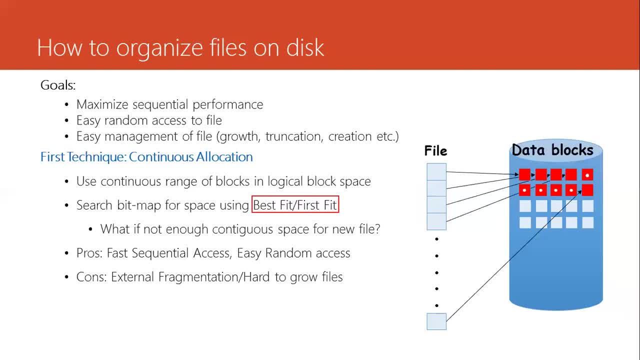 want to access. okay, the problem with this method is that it requires that the file, the size of the file, be known before we actually open it. this is the ultimate fragmentation problem that we encountered, because if the file does not fit in the available space, we need to. 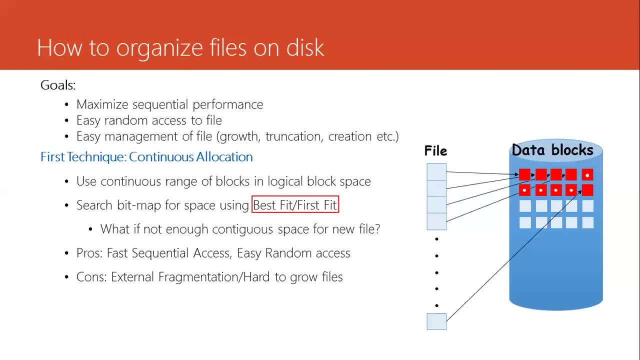 move it around right. this is basically external fragmentation, and the files are hard to grow as well, because if we grow the file more than the available space and it does not fit in the available space, we need to fit somewhere else, and that is very expensive, and also the gaps that are formed due to dislocating a 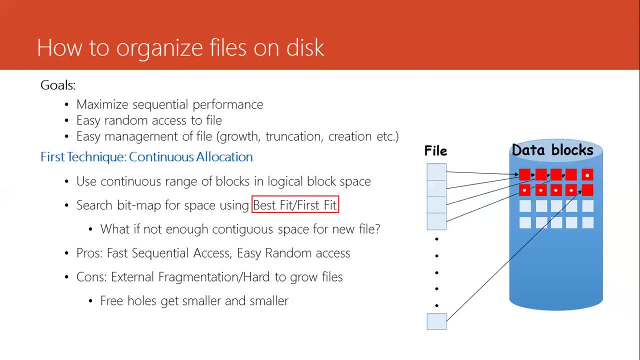 file to a large, larger range of blocks, make holes that actually get smaller and smaller as we fit more and more files into the left out holes and eventually you would have to move your data alone. okay, you could compact this space using defragmentation, but that would be very expensive. the second method of 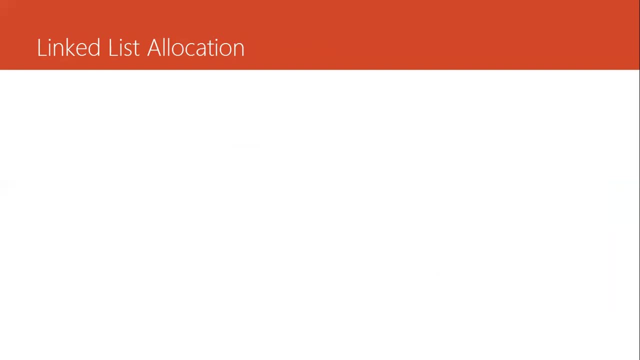 allocation is the link list approach and, as the name implies that each physical block in the disk would now contain two things: it would contain the data as well as a pointer to the next block, so the blocks would be placed in any available location and would just be linked together. the only thing is that now we 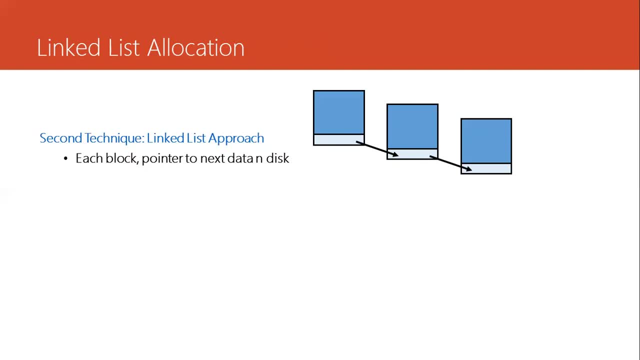 only need the address or index of the first block, or the start block, which would essentially guide us to all the other blocks. the last block must have a way to indicate the end of the file blocks, which is done through assigning pointer of the last block to a null value or a minus one value. this concept 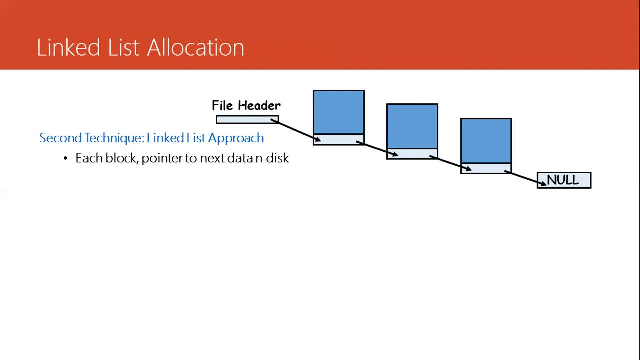 is what is called linked list, basically block allocation. the user would now be able to go to the exact location by just following these links. benefits of this method is that there would be no external fragmentation, as you can place your data anywhere you want, and it also does not have any problem with the file growth, as was the case in the contiguous. 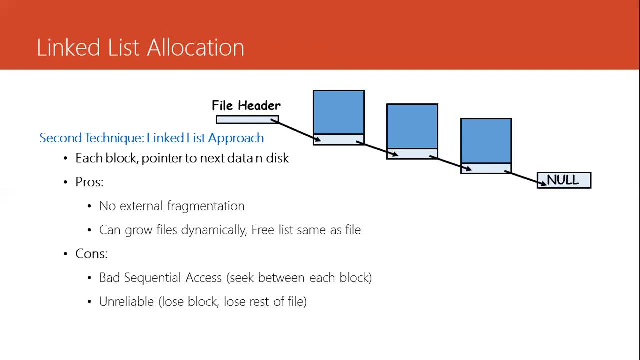 allocation method. the downsize, however, is that, in addition to the pointer overhead, it also requires large seek time, or in other words, this method has bad response to sequential access, because you would have to traverse all the links until you reach the point or the blocks that you require. this method is also unreliable because 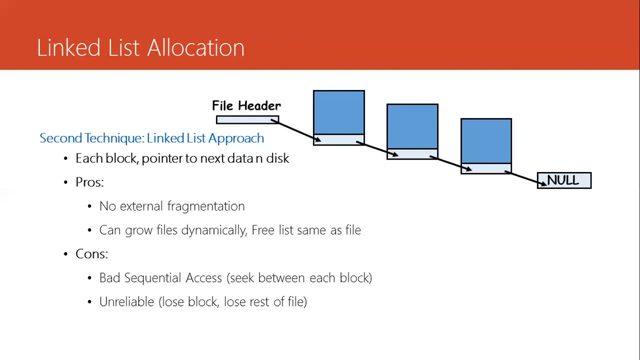 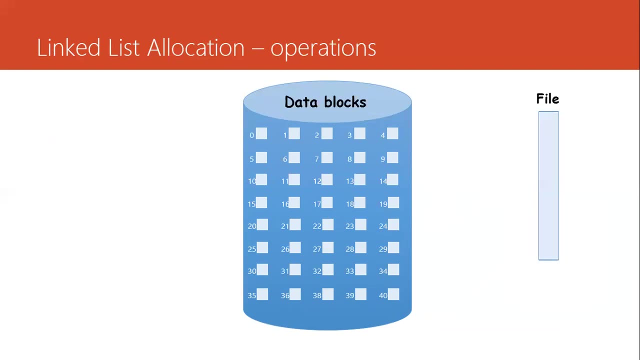 you lose a block, you lose all the PI. okay, and the random access is very expensive, especially if the linked list is not cast in the DM some operations that the linked list can perform. so we have this file, we break it down into logical blocks and we are actually linking all the blocks in an orderly. 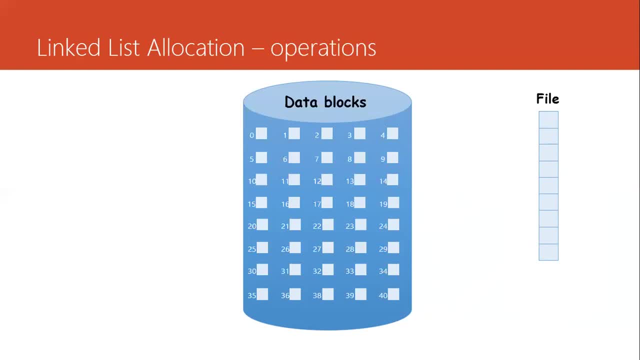 fashion in the disk drive that follows each other until the end of the file marked with a null value. right? so when we create a file, we are basically performing this: these block is linked through the previous block until the null value is reached and assume that the adjacent blocks are not free, as we. 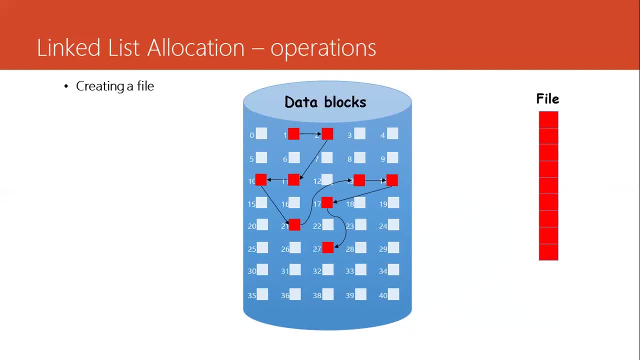 know that one of the main advantage of this method is that growing a file is easy and the blocks can be assigned any available location on the disk right. therefore, there is no external fragmentation. you just have link the new file, new blocks, and what happens when we truncate a file or in other? 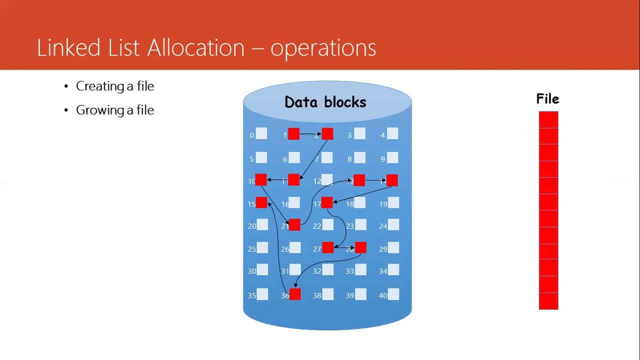 words, we delete some portion of the file. in that case you simply remove the unwanted blocks, okay, and relink the disconnected blocks. but but be careful, because if you don't do that then you will have a problem. if you don't be very careful. before we remove any block, make sure you link the desired. 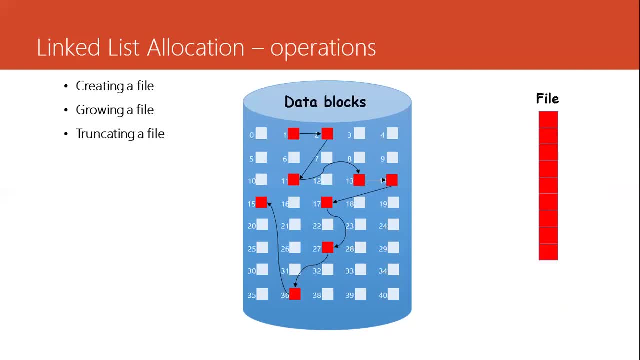 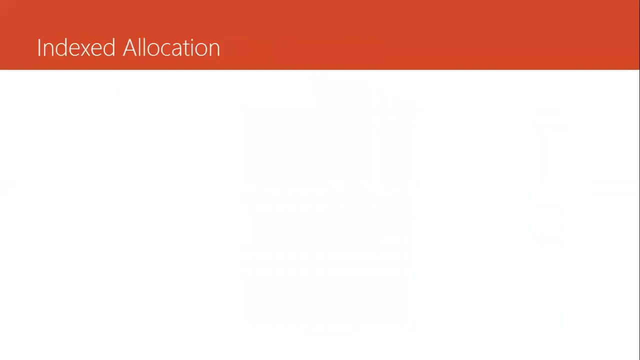 blocks first, okay. then poof and remove all the blocks, okay. in fact, do you think we really need to remove anything at all? well, no, because they are not linked and are considered free space and the file system actually provides all these operations on the files we talked about: contiguous allocation, allocation and linked list allocation. 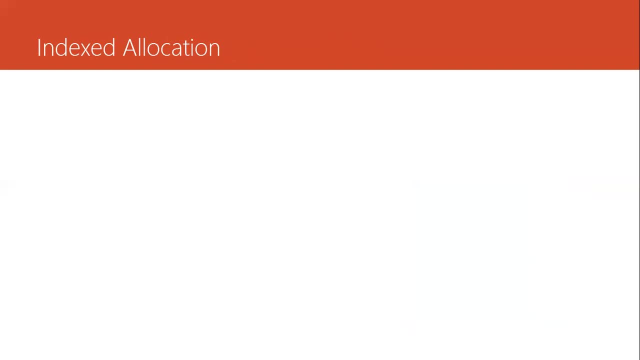 and we know what are their advantages and disadvantages. now we talk about index allocation, which is similar to a book that has the first few pages of it reserved for the index into the rest of the pages. the book here is a disk blocks and the content pages are special blocks. that has all the indexes of the file. 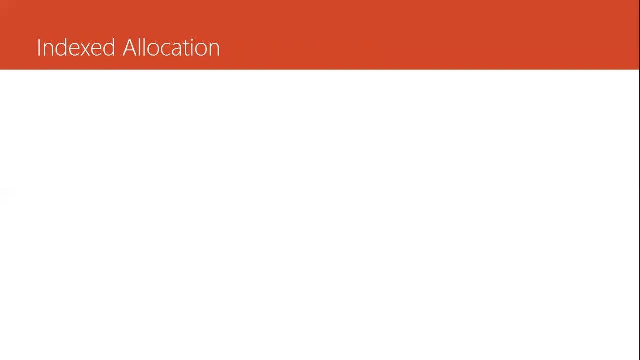 pieces. okay, we store the logical blocks in physical blocks on disk, based on the availability. so just recall that the aim is to efficiently lay out the data so that it can be pressed easily for read write operations, which are the main functions of any file system: the. the file basically resides in the directory. 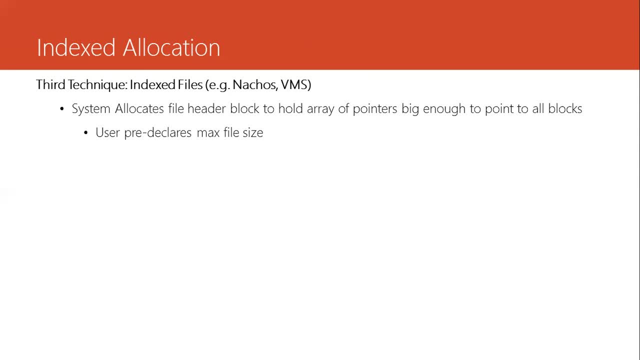 and the system gives it an index block which provides index to the blocks or fragments of a file. the user is also required to declare the maximum size of the file. what are the advantages of this method? similar to the linked list method, the index based technique has no. 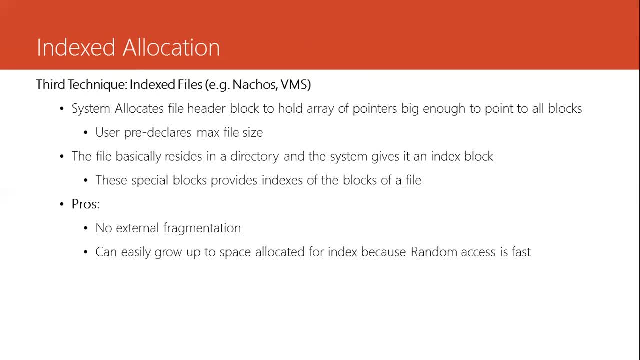 external fragmentation because the blocks can be allocated to any available location and the response to file growth or file shrinking is improved, as in the case of file growth. truncate search in the linked list case it does not have to traverse all the links until the end of and to append. 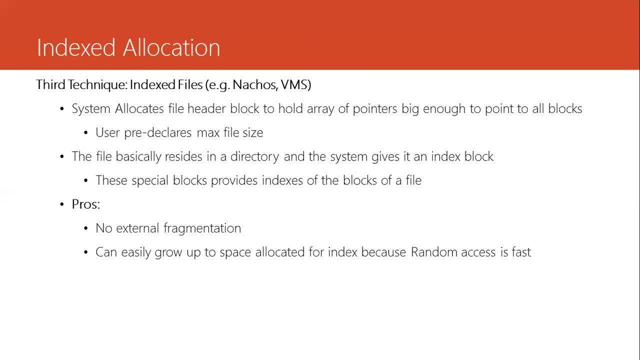 or remove any blocks, because all of these operations is dependent on random access. that is improved in the index based allocation method. now we can jump directly towards the location based on the index of the required blocks. the obvious this advantage of this method is the expensive overhead of intensive use of 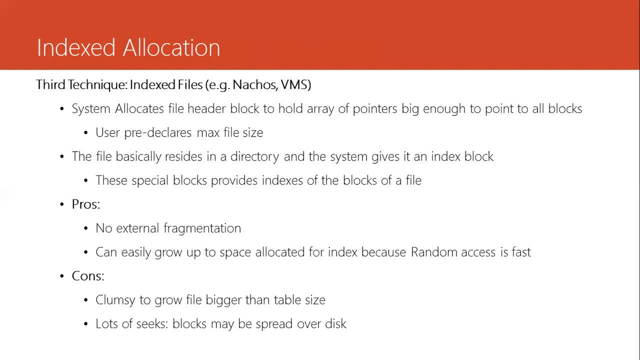 pointers to point towards the blocks of the files. and if the file is larger than what a single block can hold, then we need multi index, multilevel index for big files. if you recall that most of the disk space is eaten up by real big files, this is because if the file is big enough, 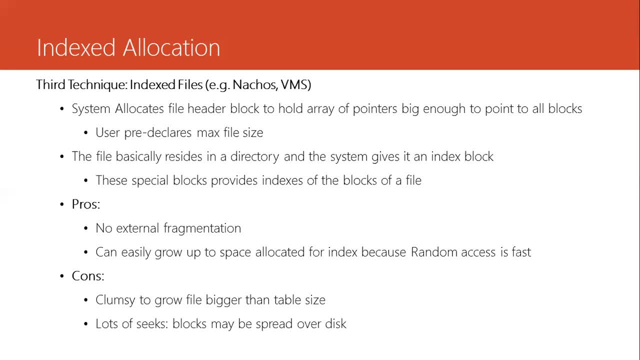 that one one blog could not hold all the indexes of the file, we would require multiple blocks to keep track of this file, and the searching could also become quite complex, as a real example of this is the unix operating system that uses an inode number that is based on multi-index structure to support large 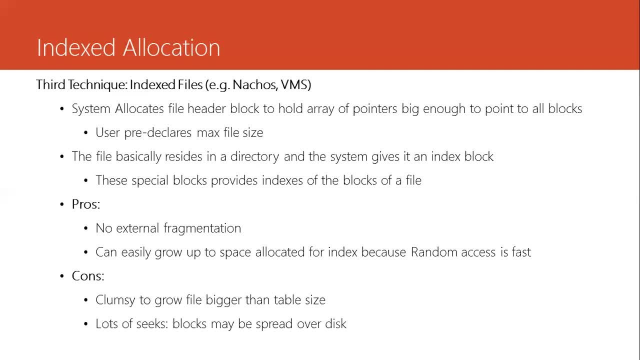 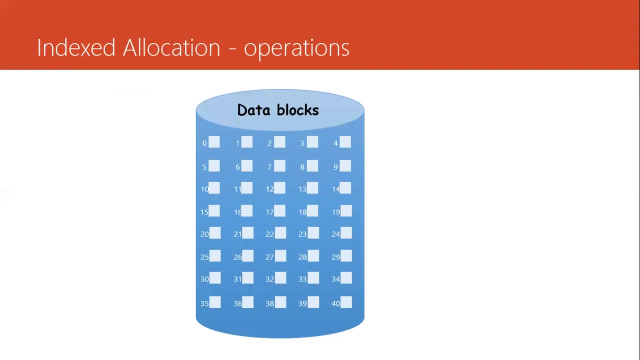 files and, due to the spread of file blocks over the disk, access to to the file requires a lot of seek time as well. so, uh, these are uh some of the operations that uh the index based allocation method supports. so what happens when we create a file? it is assigned an index number block. okay, 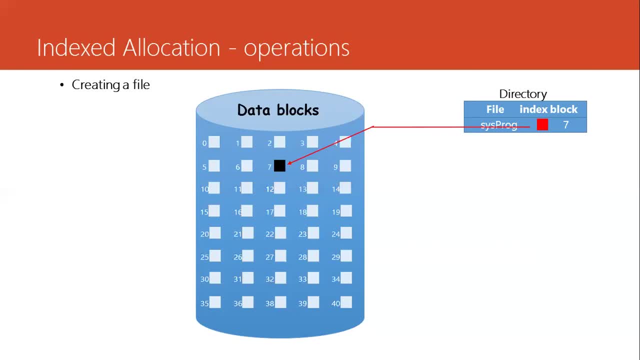 the file is actually residing in the directory and it is assigned an index block number which identifies the special block in the disk drive that has information into all the indexes of the blocks of the sysprog. okay, and any free space on this can be allocated to the blocks of the data. 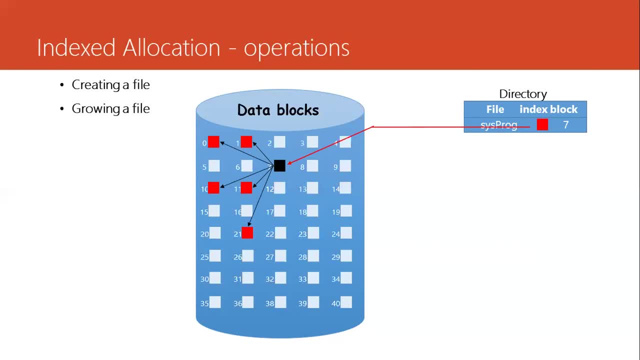 and what happens if the user increases the size of the file. the user grows the file. simply. the new blocks are allocated any available space and the entries of their indexes are updated in the index block, which is the special block assigned to the sysprog at the time of. 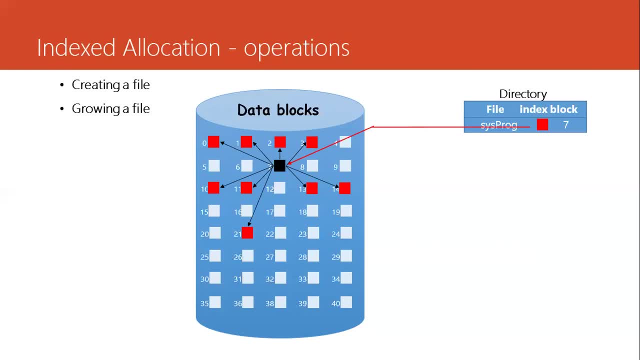 creating the file. so you can see that there is no external fragmentation. and what happens when we truncate a file, or in other words, delete some portion of a file? well, in that case, you simply need to update the index block. you simply remove the indexes to the unwanted. 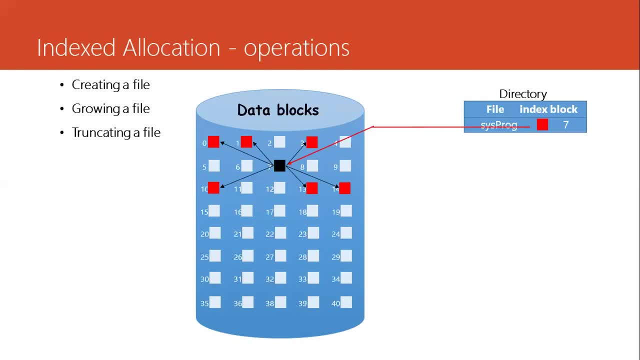 blocks and replace it with minus one. okay, what if we create a new file that is named assembly? the same process is going to repeat. the file is assigned an index number that has all the index information to this file. so, uh, what is this special block? well, this special block looks something.